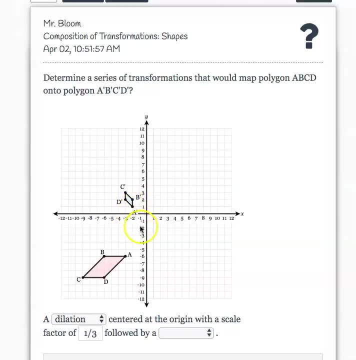 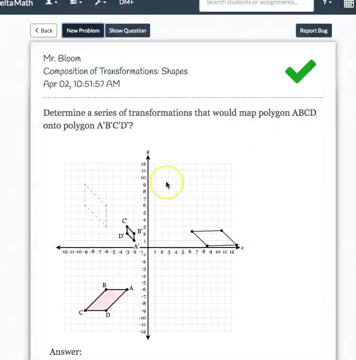 And that's going to be two, one up here And that's a 90 degree rotation, clockwise. But I've got to do a 90 degree rotation counterclockwise because it's counterclockwise, So that means 270.. Okay, So now, as I cursor this up and submit my answer and I say, yes, oh gosh, we're right, And they're going to show us what's going on, So it's there, And then it's a third the size. 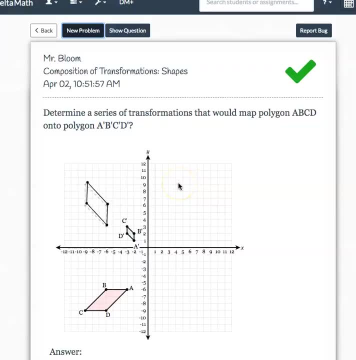 Okay. So we have to be thinking. there's two compositions that are going on with this. This one's a tougher one, And how did I know it was going to be a rotation of 90 degrees? say, well, those are the only rotations we have. But the big thing is, corresponding sides were perpendicular to each other. Okay, And that's how I knew that they'd have to be a rotation. If I have a reflection, corresponding sides, you know I can see. 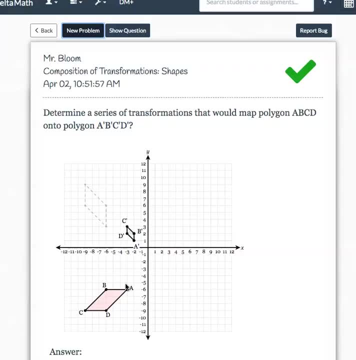 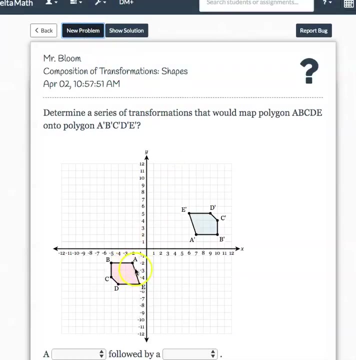 the corresponding points beyond a line perpendicular to them. If I'm looking at a translation, corresponding sides are parallel to each other. So those are the things I'm thinking about when I do this. Let's go on to another problem Now. on this problem, it appears that the shapes are the same. Okay, and I'm going to check. I'm not going to guess: de 123, de 123. So the shapes are the same. So this is an isometric translation. 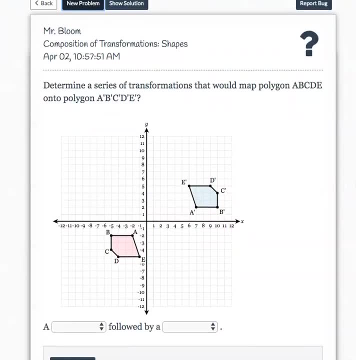 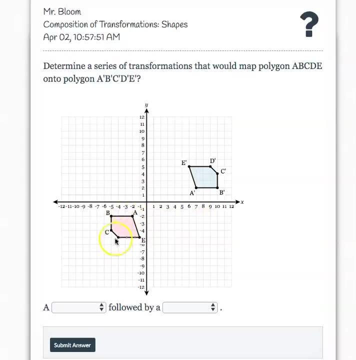 There's no dilation involved in this. So now when I'm looking at this, I'm going to go. well, I could just slide this over, But you see how this orientation is different from this orientation. This looks like it's going to be 180 degree rotation, Okay, and then a translation, And let's talk about that. If I go 180 degrees from here, I'm going to be up here with a okay. 180 degrees from here, from E, I'm going to be here. So that seems to make sense. 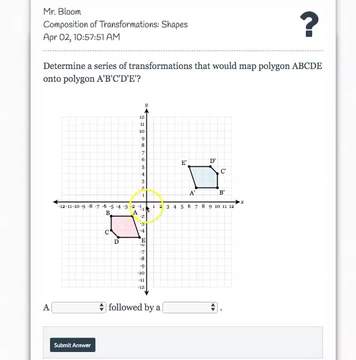 I'm going to make it okay, All right, but 180 if E is at negative one negative five negative one negative five times negative one, which is one, five. one, one, two, three, four, five, I'd be right here. I just have to translate E: one, two, three, four, five units, So it's 180 degree rotation, Okay, and I don't have to go clockwise or counterclockwise with that, doesn't matter, it's going to end up the same. And then I'm going to do a translation because I'm going to slide it over. 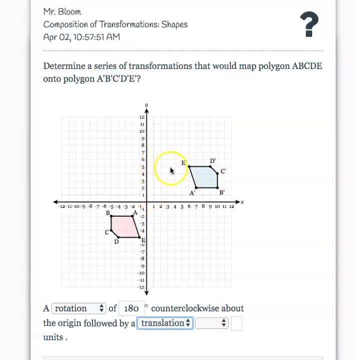 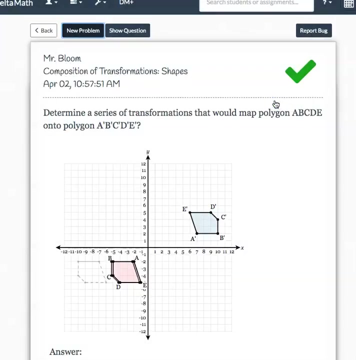 So it's going to go from here: one, two, three, four, five, And I'm going to go to the right five units. Okay, now I've got to get my submit button and hit yes, And we'll watch what happens. 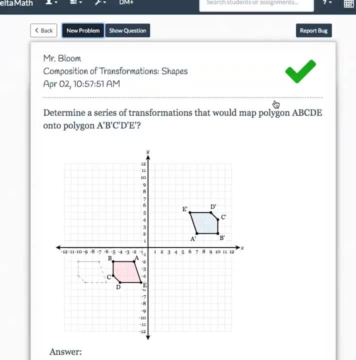 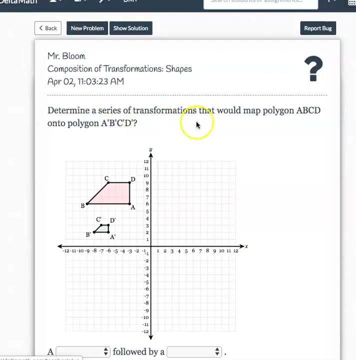 They went left five units and then rotated. but right that rotating and then going right five units, we'll do the same thing. Okay, Now new prop: determine a series of transformations that would map polygon ABCD onto polygon A prime, B prime, C prime. this is a dilation first, So it's 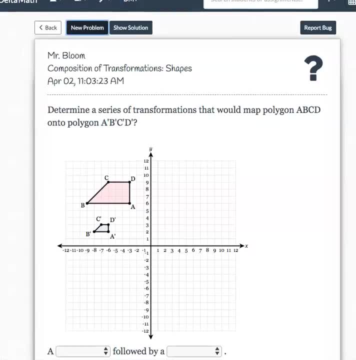 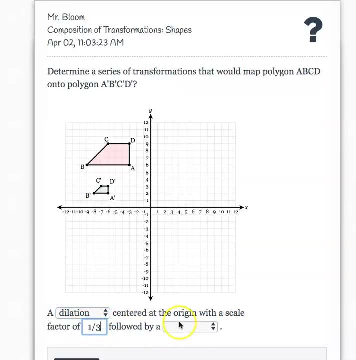 going to be a three to a one, So it's a third the size. Okay, that's my first thing. Okay, now that's going to shrink this down and it's going to be a three to a one, So it's going to be a third the size, a third the distance. this is three out, and this is one, two, three, four, five, six up. So now a third of three is one, And remember it was two, So it's I'm at one, two. And now this is my new a spot right here at negative one, two, And I'm going to go one, two, three, four, five units to the left. I'm going from a to a prime, So my left translating five units. 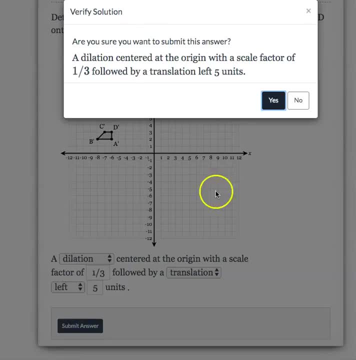 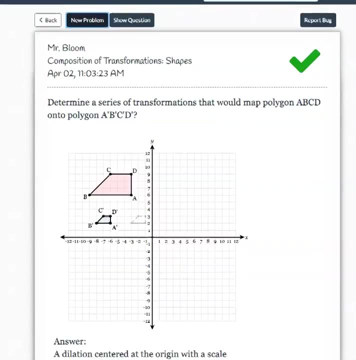 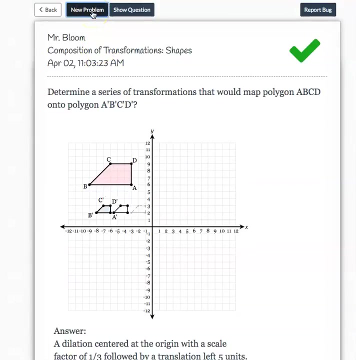 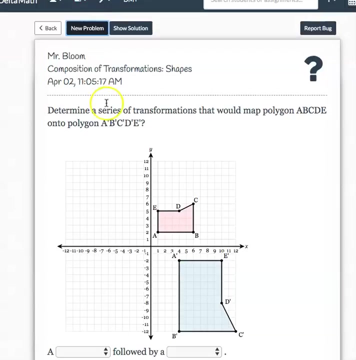 Okay, now submit my answer. And I seem to be right now. every time I answer whether I'm right or not. Oh, nope, I should say I'm gonna. we're gonna get the next one wrong. I want to show you something. Okay, first of all, we'll do the right question. then I want to make sure you understand that there is a solution to this. So I got a new problem, All right, So this one is another transformation, That's a dilation. first, 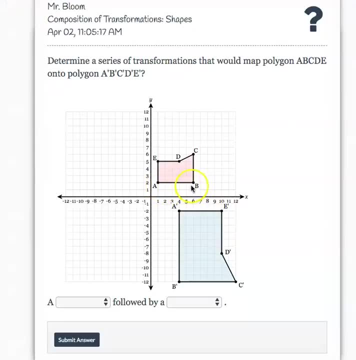 So I've got one, two, three, four, five of my original, or six, excuse me, five length on my original, And then from a to b, I'm going from two to 12.. So it's 10.. So it's twice as big. Okay, so it's a dilation That's twice as big. Now, since it's twice as big, you got to keep in mind what's happening. But they'll do, probably. and then, if it's twice as big, twice as big is that it's going to be here And this can be here. So my new a is up here. 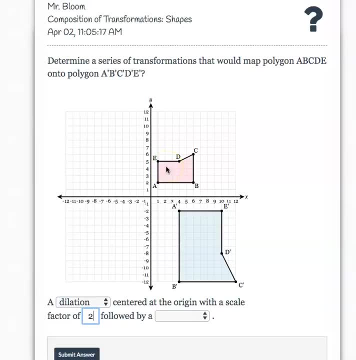 At two, four and now a 90 degree counterclockwise rotation. Now, excuse me, a clockwise. Yeah, 90 degree clockwise would bring it to the original, But we're doing counterclockwise, So it'll be a 270 rotation. If I want to do a rotation, it'll be a 270 to do this one correctly. But remember, we said we're going to do this wrong, So let's say it's 90. Because you know that that's really what's going to be. But 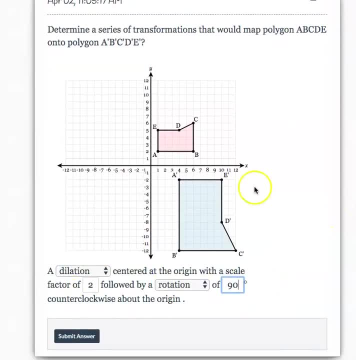 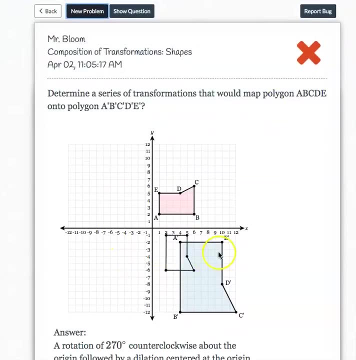 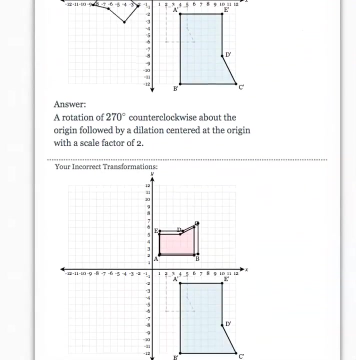 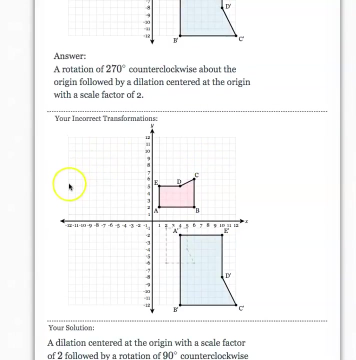 if I put this in. okay, if it's counterclockwise, this is not counterclockwise. I just want to make sure you see what happens when you're wrong. So we go down and we see, oh, there's that 270.. And they'll do the rotation and then they'll grow in, And we did the shrink and rotation first. So they'll do this And they'll do the. that's 90 degrees. That's what our answer was, And so 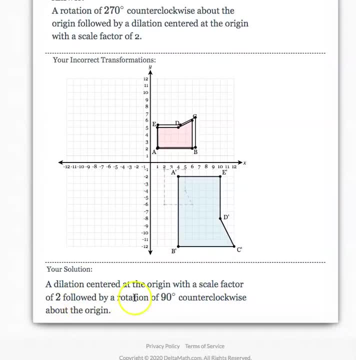 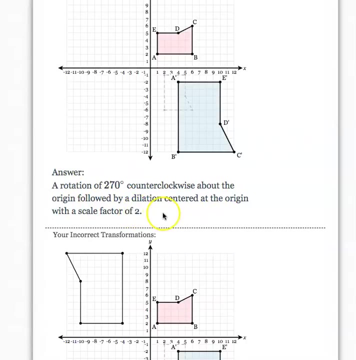 the dilation centered at the origin, with the scale factor of two followed by rotation 90, counterclockwise about the origin is: does this Okay? so they're actually showing us where our piece would have been And we are looking here at a rotation of 270.. Like we talked about, with a dilation of two, but we could have flip flop those. we could have had it grow and then done the rotation, or done the rotation and then had it grow. Okay, Now, that way you can see both things and see what's happening. Let's do one more problem. 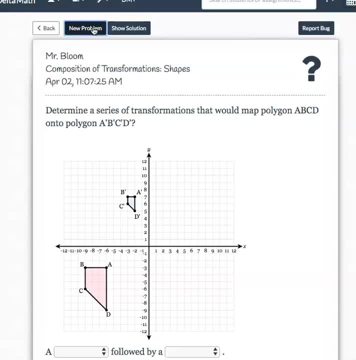 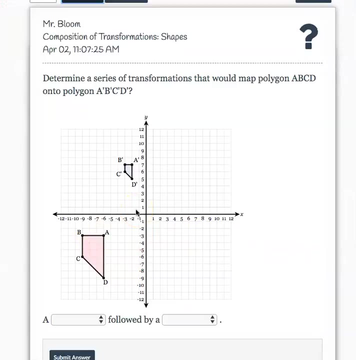 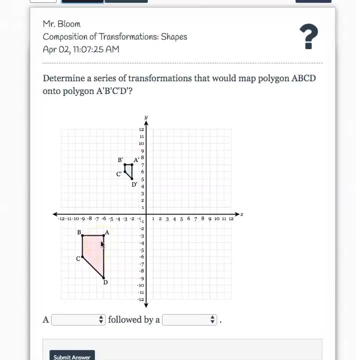 And up you know down three down you know out six down three. A third of those is out two down one. So I'm here, So my A will be right here and I'm going to slide it up to this position. 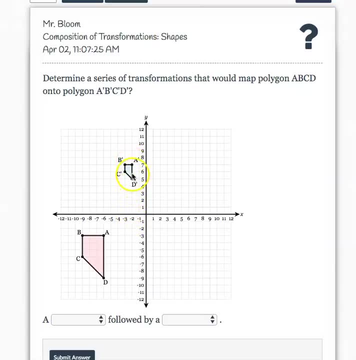 So it's going to go one, two, three, four, five, six, seven, eight. So I'm going to shrink it, dilate one third And I'm going to translate it up eight units And we're going to go ahead and get that done with a submission. 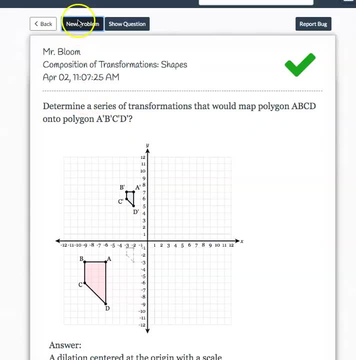 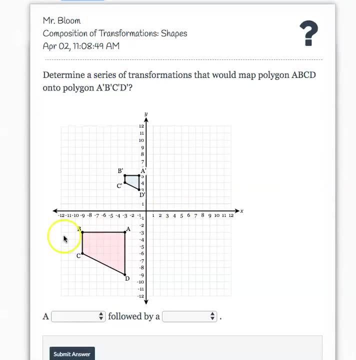 Okay, so we see our submission And we still have 30 seconds on the 10-minute video, so let's try one more Again. this is one very similar to the one we just did. Okay, I'm going to shrink this down. 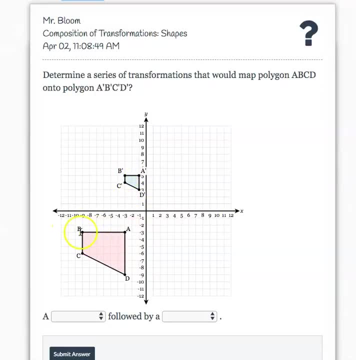 And why am I just going to shrink it? See how A, B and A B are parallel to each other. This means I'm translating because they're going to be parallel to each other. There isn't a rotation involved or a reflection, because they're in the same orientation. 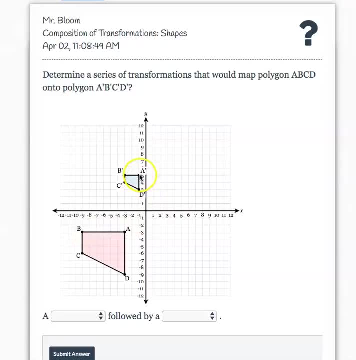 So I'm going to shrink it by how much: A D is two And A prime- D prime, I should say- And A D is one, two, three, four, five, six. So I'm cutting this. 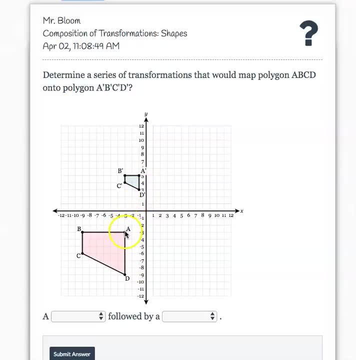 Boy, I'm cutting it by a third. Okay, so I'm bringing this The A's at three, three Negative, three, negative three, And I'm going to bring it down to negative one- negative one- by multiplying by a third. 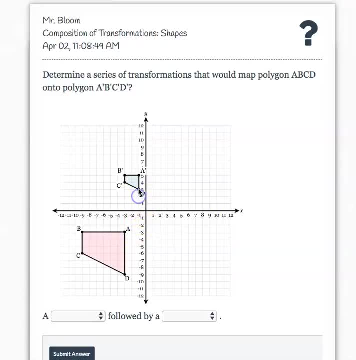 And then I'm going to slide it up. one, two, three, four, five, six units up. So I'm going to dilate one divided by three And slide it up. How many units did we say Six? So we're going to translate it up.